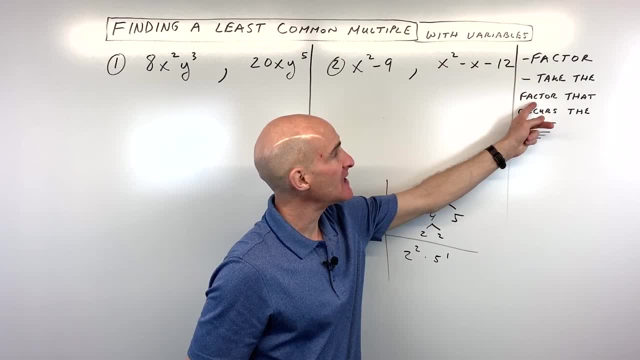 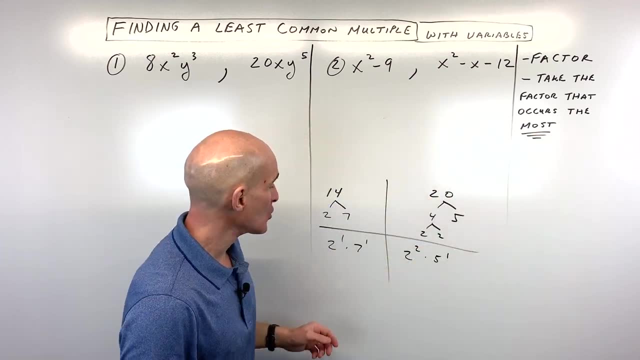 common multiple is. follow these steps: First factor, then take the factor that occurs not the least. it's called the least common multiple, but we want to take the one that occurs the most. So here you can see, we've got 1, 2,, 2, 2's, so we're going to take the one that 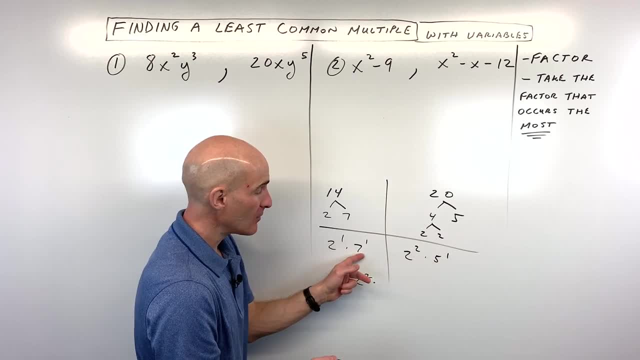 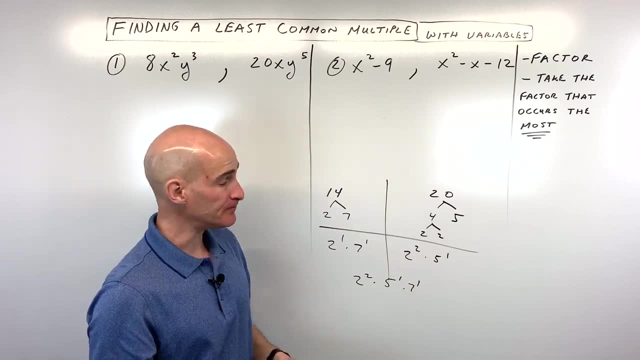 occurs more 2, 2's. Here we have 1, 5, no 5's, so we're going to want to take 1, 5, 1, 7, no 7's. we're going to want to take the one that occurs more 1, 7.. Now, if we multiply these together, 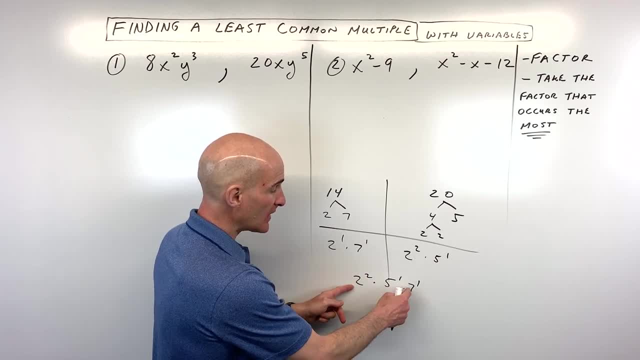 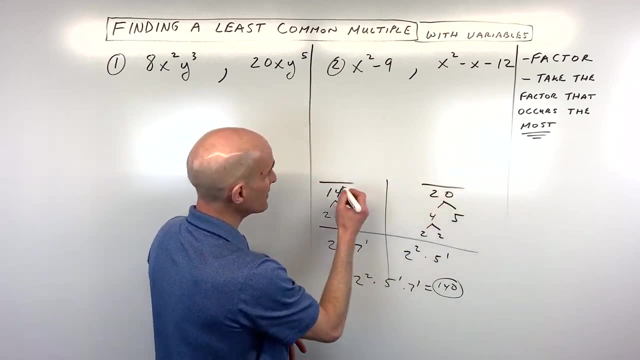 we've got: 2 squared is 4, times 5 is 20, times 7 is 140.. So what that means is now is that imagine if we had two fractions like this. Say, there was a numerator here and we said: 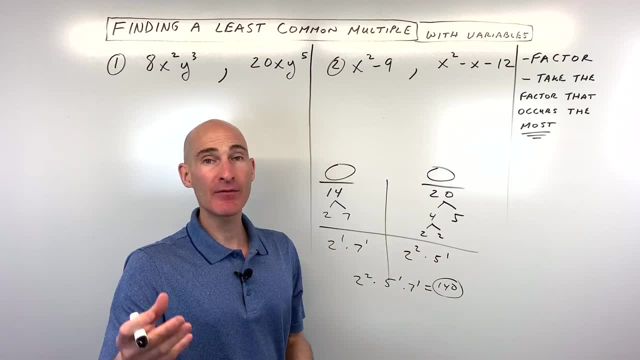 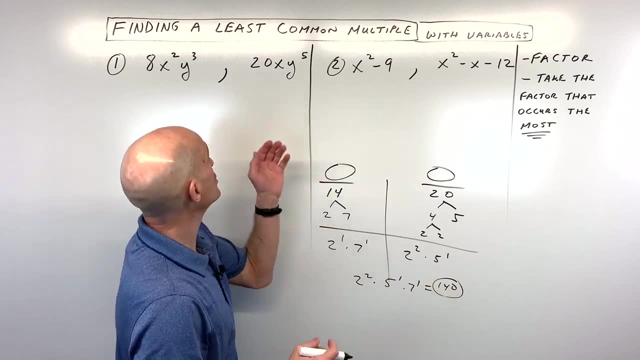 oh, I want to get a common denominator. That common denominator, that smallest denominator that we could find, where 14 would go in too evenly, 20 would go in too evenly, would be 140.. Okay, so let's jump over to example one. So what we're going to do here is we're going to look at 8.. 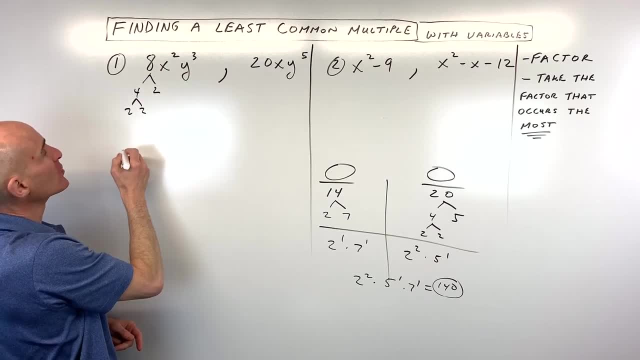 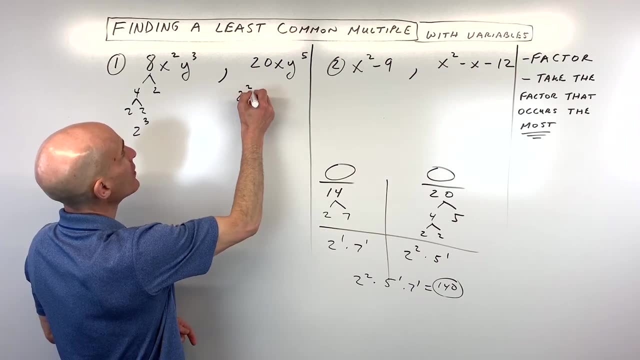 8 is really like 4 times 2 and 4 is 2 times 2.. So you can see this is really like 2 cubed And 20. we already did that over here. that's 2 squared times 5 to the first. So we want to take what occurs the most. We've got three 2's here. 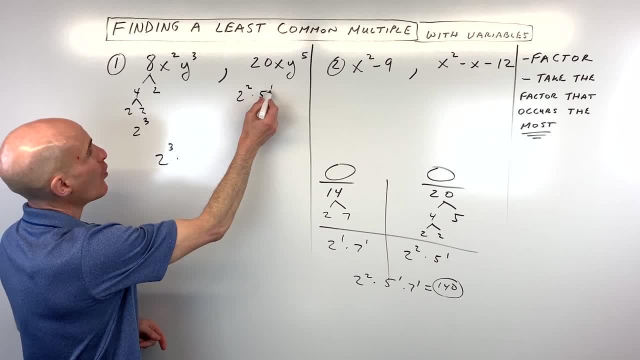 two 2's. here we're going to need three 2's. We're going to need 1- 5, there's no 5's here, And here we've got x squared, that's like two x's multiplied together. Here we have one x. 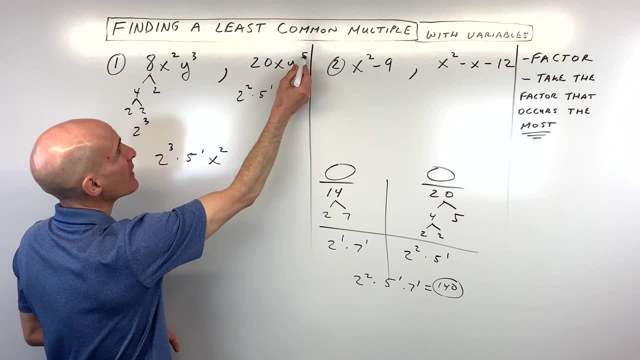 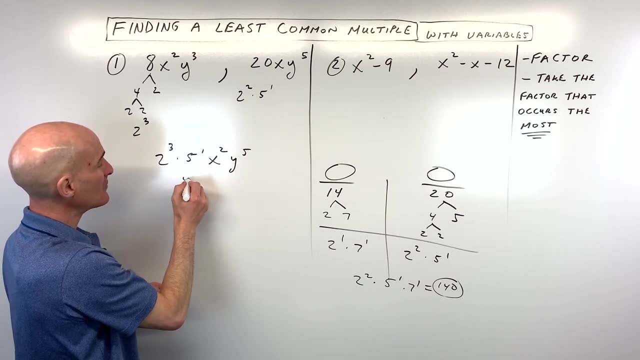 we're going to take the one that occurs more. Here we have three y's, here we have five y's. we're going to take the one that occurs more. So if we multiply this together, 2 cubed is 2 times 2. times 2, which is 8, times 5, is 40, x squared y to the fifth and that's going to be. 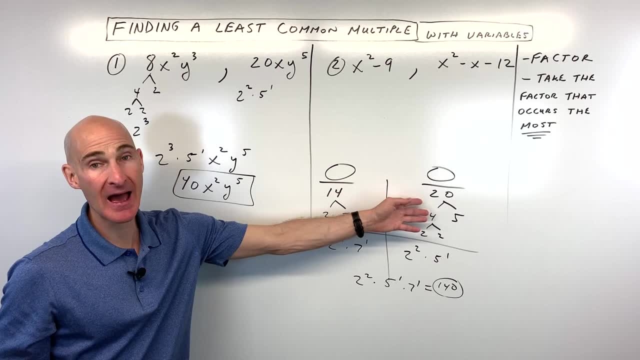 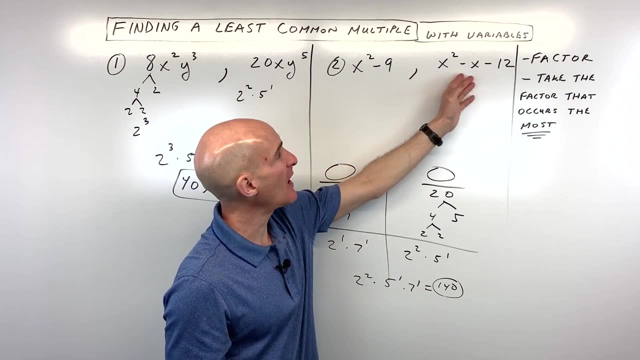 your least common multiple, Or if you're thinking about finding a common denominator, that's like your lowest common denominator. Now for number two. this one's a little bit more challenging, because what we have to do is we have to see these are monomials like one group. This is 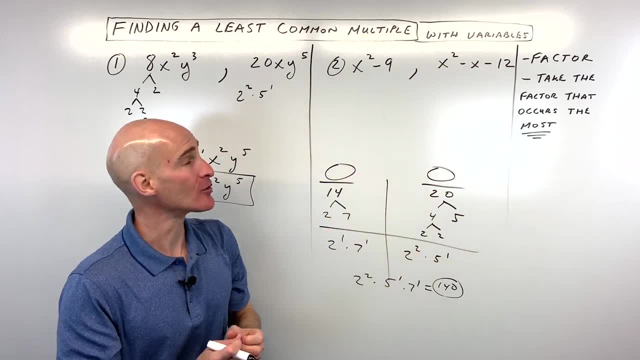 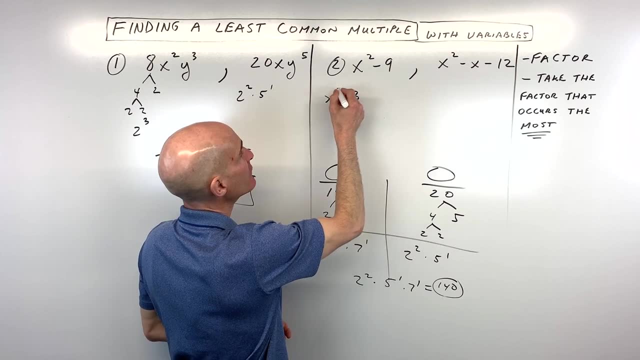 a binomial, this is a trinomial. What we want to do is we want to factor and see what this is made up of. So x squared minus 9, this is what's called a difference of two squares, And you can factor it. 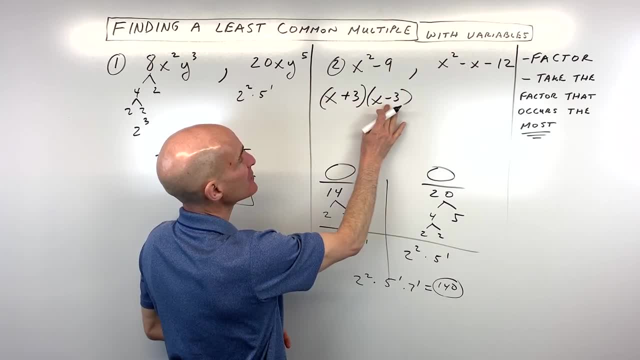 as a sum and difference pattern: See sum is add, difference is subtract. So x plus 1 is minus 9, plus 3 times x minus 3 gives us back x squared minus 9.. Over here we have a trinomial with a. 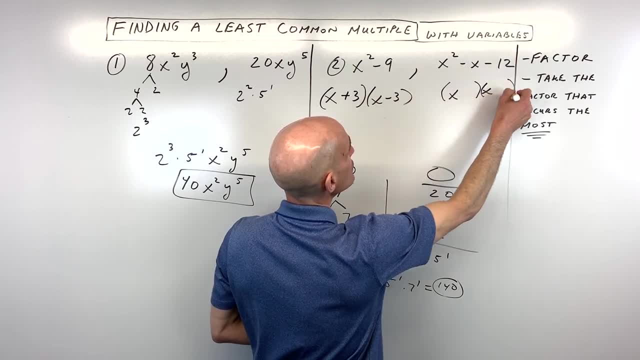 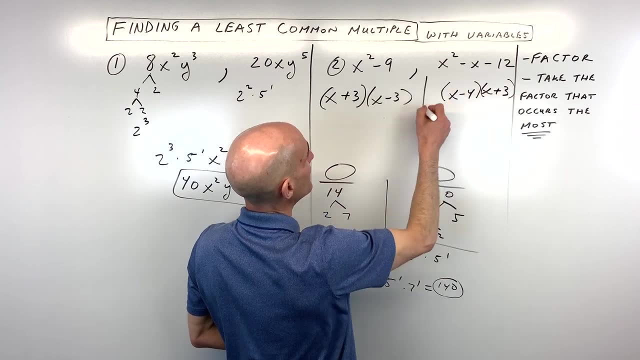 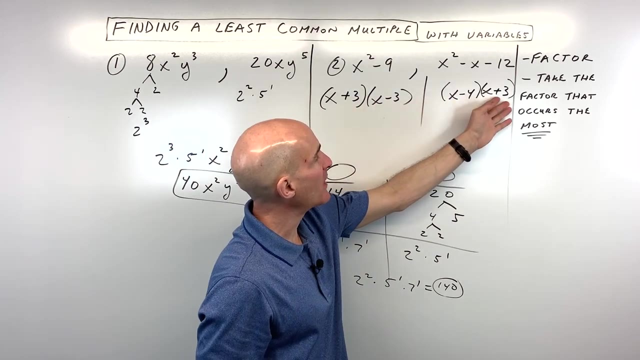 leading coefficient of 1.. We just have to ask ourselves what two numbers multiply to negative 12, but add to negative 1? That's going to be negative 4 and positive 3.. Now here's where we want to take whatever occurs the most right, So we can say: well, we've got 1x plus 3, 1x plus 3,. 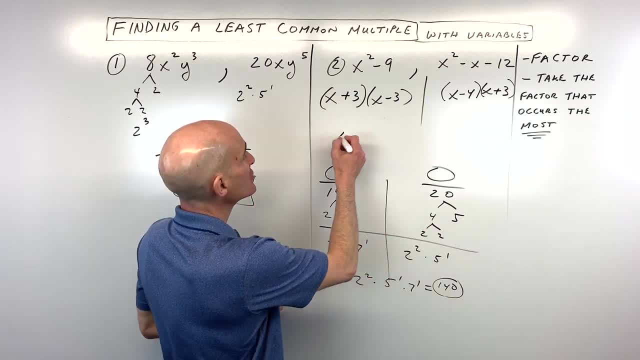 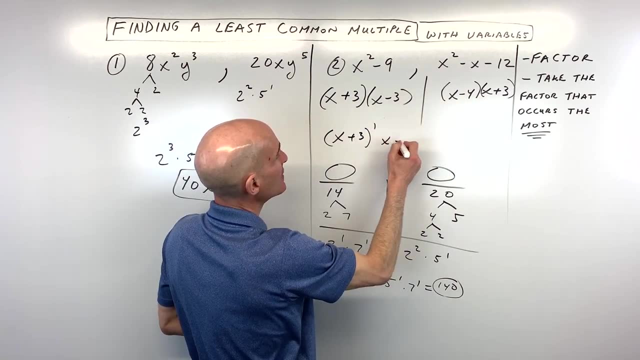 it's a tie. What do you do in that situation? Well, you're just going to need one of those, okay, So just a tie for 1 there. Here we have an x minus 3, no x minus 3.. We're going to need 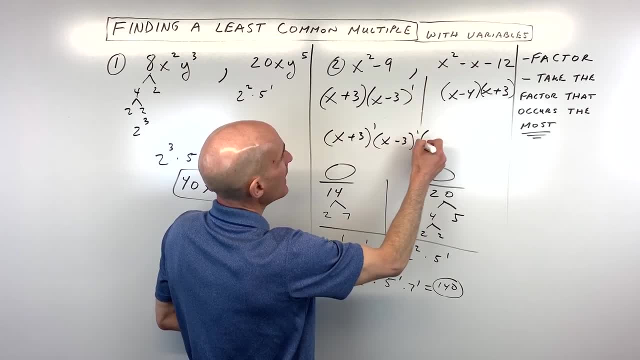 whichever one occurs the most, which you can see. there's 1 here, so that's 1.. And then we have an x minus 4, no x minus 4, we need 1x minus 4.. Now, I don't have to write these ones here, because 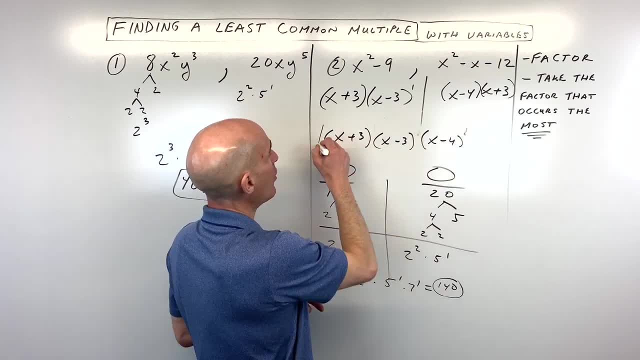 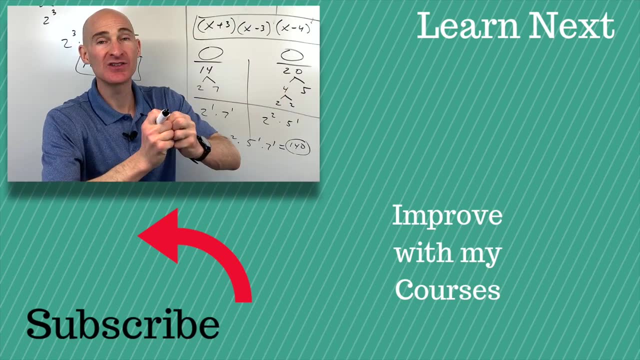 anything to the first power is itself. But just to show you, all these multiplied together represents the lowest common multiple or the common denominator, if you're trying to combine these into like a fraction with a common denominator. If you want to see how to apply this least common. 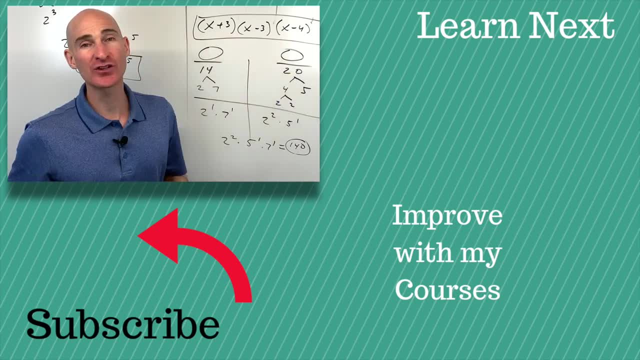 multiple to finding common denominators and combining rational expressions, adding and subtracting. follow me over to that video right there and we'll dive into some more examples. I'll see you in that video. 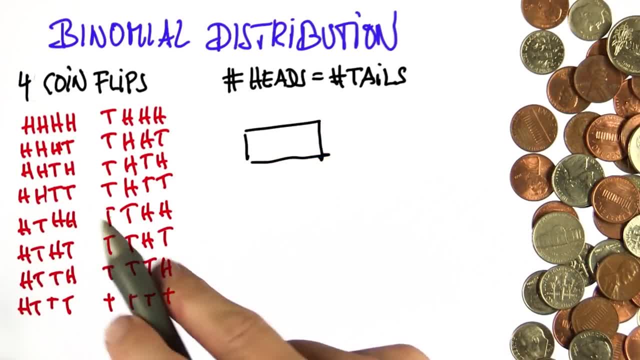 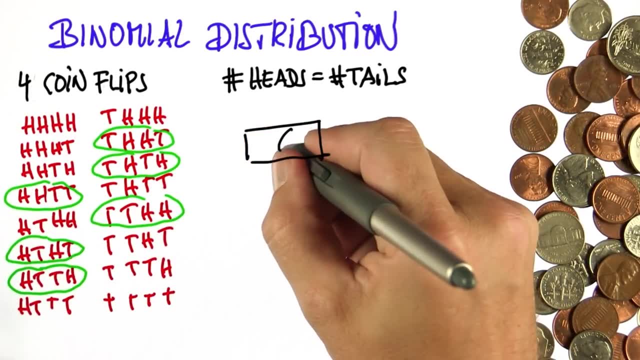 And going through the truth table is a bit more painful, So let's find the one where the number of tails and heads are the same: Those 3 on the left side and those 3 on the right side, for a total of 6..